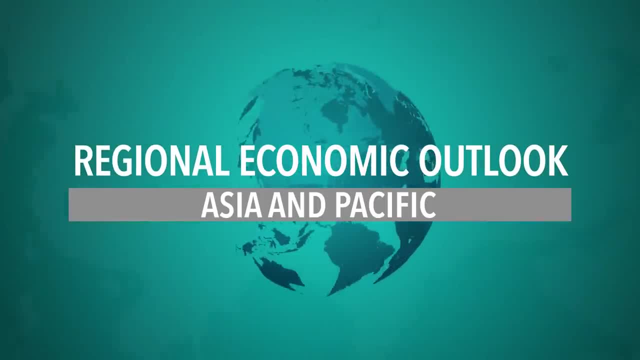 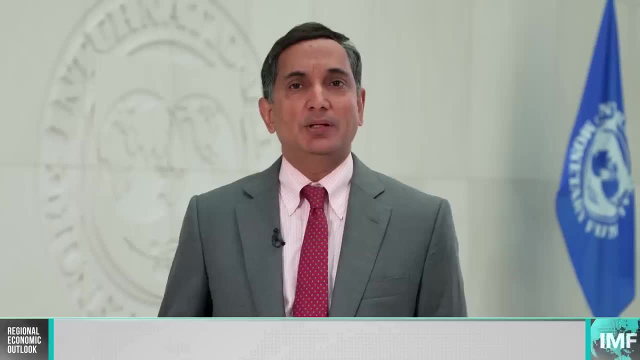 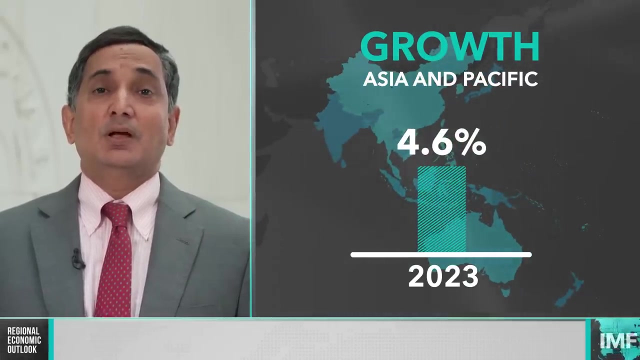 Asia remains a relatively bright spot, accounting for about two-thirds of global growth in 2023, well above its weight in the world economy. Growth in 2023 is projected at 4.6 percent. This is due to stronger than expected performance of China, Japan and India in the first half of. 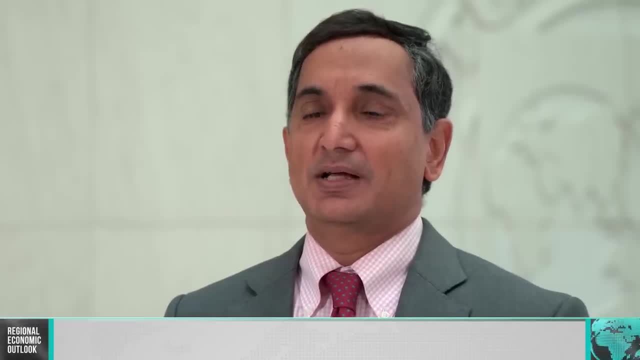 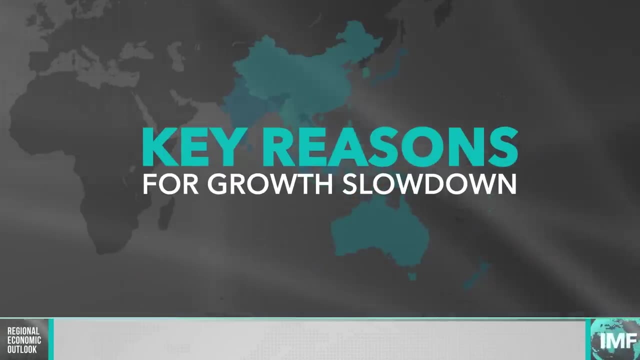 the year. Inflation is also falling faster in Asia-Pacific than in other parts of the world, But we are seeing signs of growth slowing into 2024.. Why is that? There are three key reasons. First, the world economy is slowing down and global demand is rotating towards services. 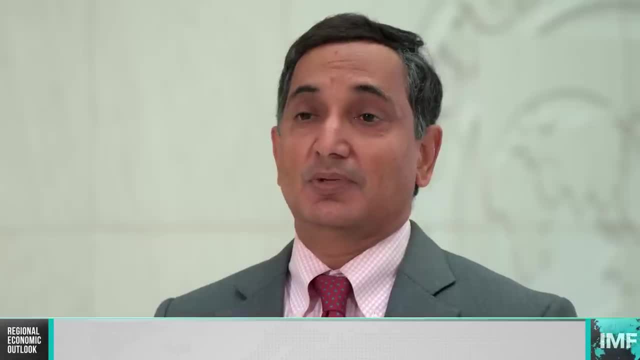 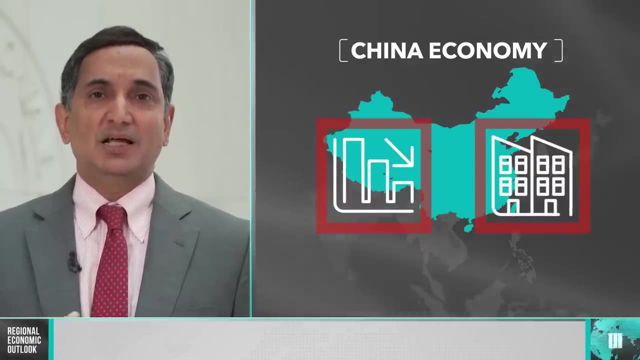 both of which imply less demand for Asia's exports. Second, China, the region's powerhouse is losing steam as its post-pandemic economic boost fades and weakness in the property sector is greater than anticipated. And third, the post-pandemic boost of domestic demand. 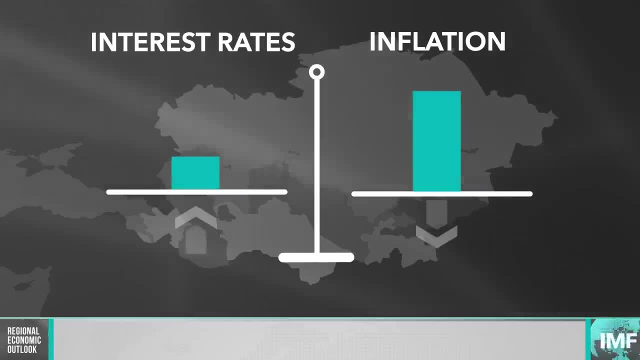 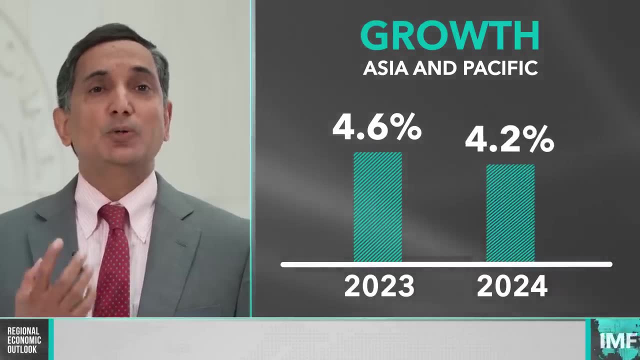 is also slowing down and global demand is rotating towards services, Also fading elsewhere in the region and monetary policy tightening in some countries has started to weigh on demand. Growth in 2024 is therefore projected to slow to 4.2 percent and risks to the outlook are to the downside, albeit more balanced than before. 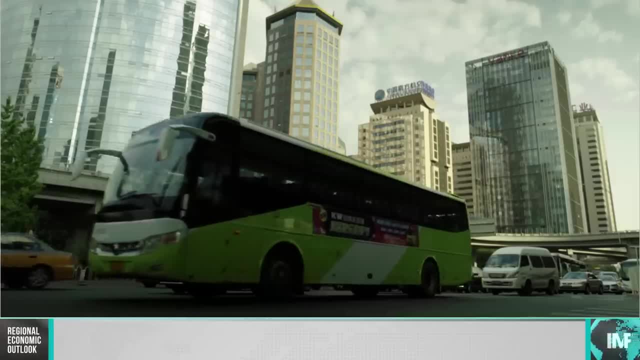 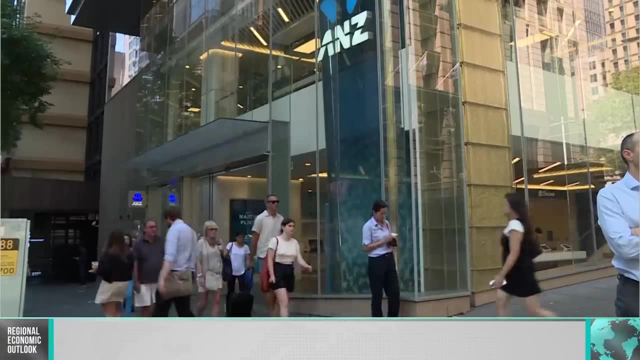 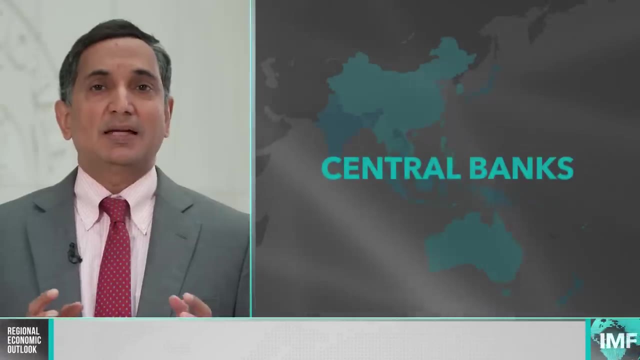 In particular, a deeper real estate problem will further slow China's growth. There could be an abrupt tightening of financial conditions, and rising geoeconomic tensions could hurt trade and investments in the region. So what does this mean for policies? Central banks need to maintain a restrictive monetary stance. 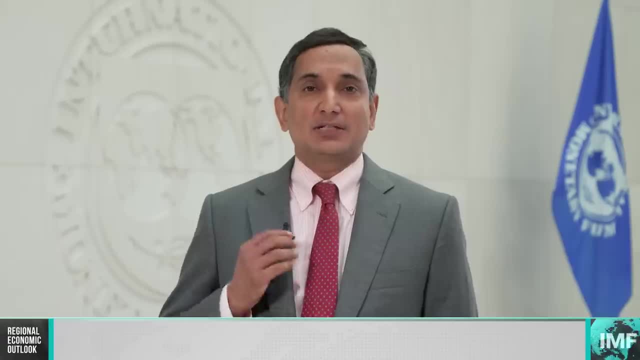 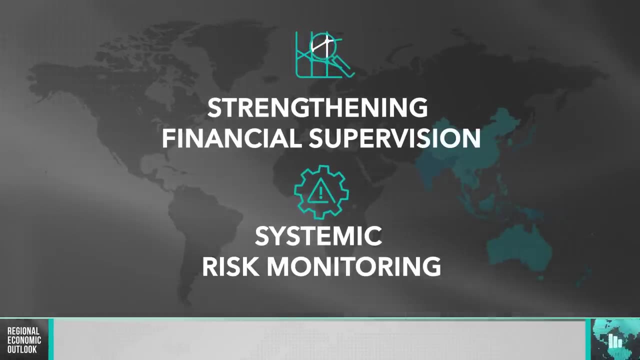 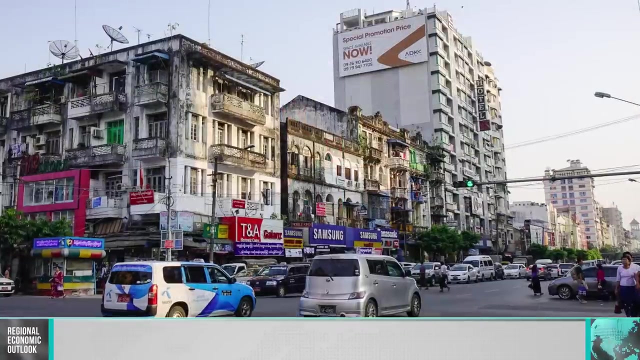 until inflation is durably at target. Since tight monetary conditions continue to pose risks to financial stability, strengthening financial supervision and systemic risk monitoring is warranted, along with the strengthening of resolution frameworks. There's a need to rebuild fiscal buffers and reduce debt levels by fiscal tightening, while providing targeted support for 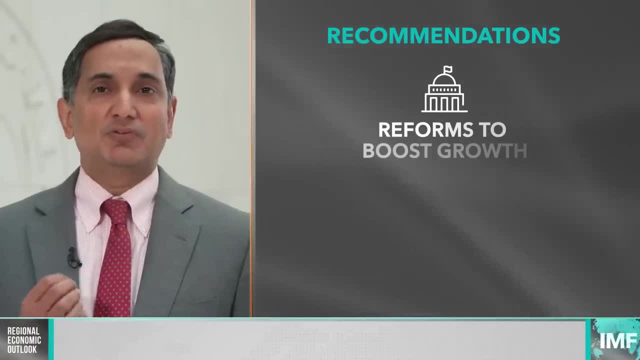 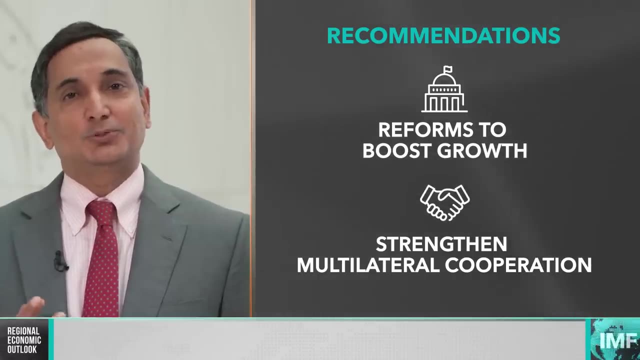 the vulnerable. Beyond these, the implementation of reforms that boost growth potential and strengthen multilateral cooperation remains vital for Asia's long-term prosperity.